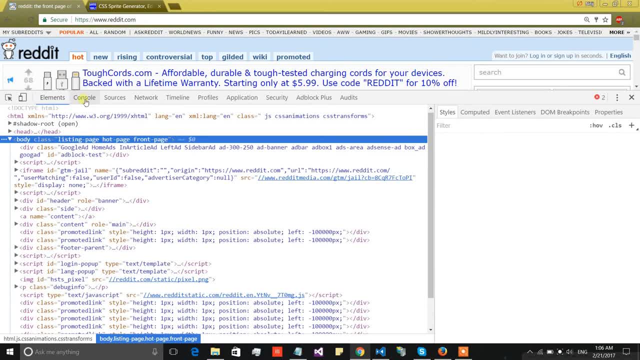 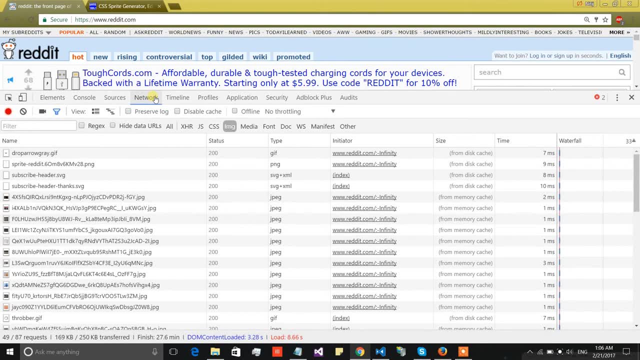 can see all the HTML elements in this element pane. we can see the console, etc. and there is a network pane too. if you have never worked or used this network pane, then this pane or window is simply to monitor the network traffic originating while we are loading any web page. so over here I have opened the redditcom website, which is a, which is a website. 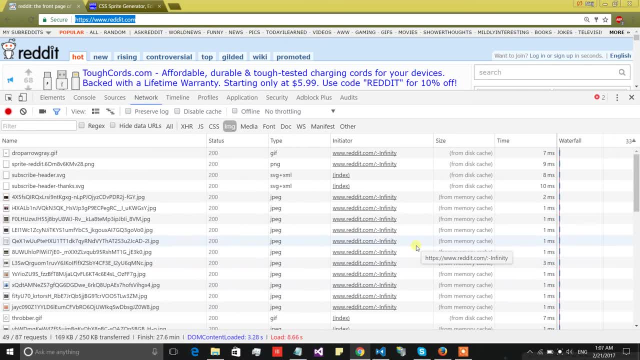 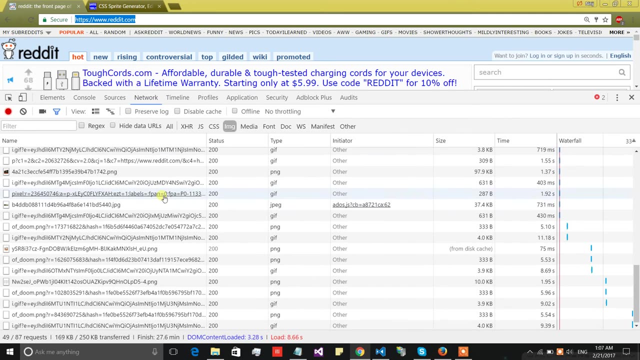 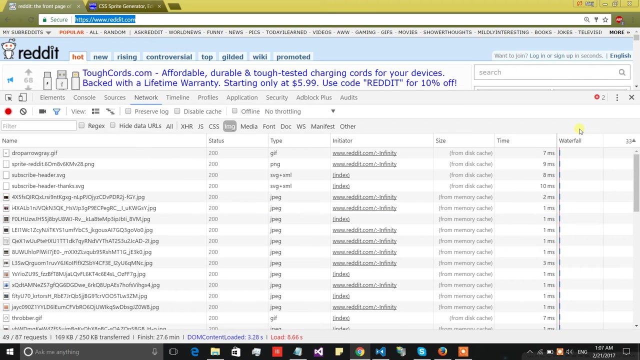 for social interactions and, as you can see in this, in this network pane, there is the network traffic recorded for all the resources. there are several different images and some different files and some js2, I think. so on the far right there is a waterfall tab which lists every request being. 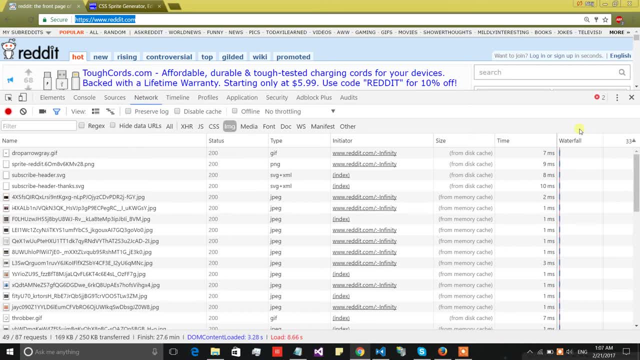 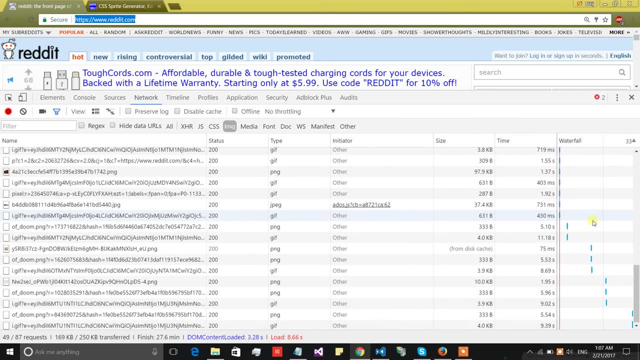 initiated by the browser in a waterfall kind of way. so it is in this way because the colored bars are moving towards the right side, based on the time taken by them to be fetched from the server, and some requests are being sent to the server and some requests are being sent to the server. 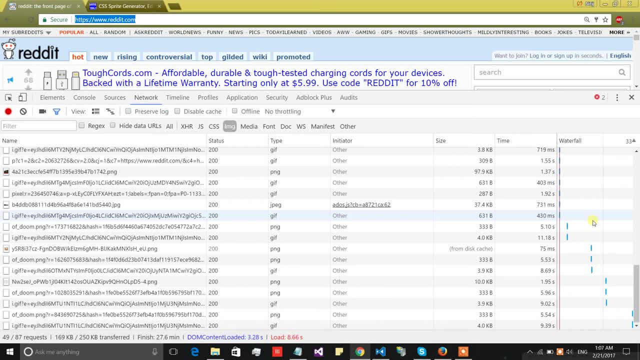 and some requests are simultaneous, depending on the number of parallel connections which are supported by the browser, and if you will hover your mouse over any request, then you can see that the actual time to download any, any resource or any component is much lesser than other things like dns lookup or initial connection or encryption, depending on the, depending if the 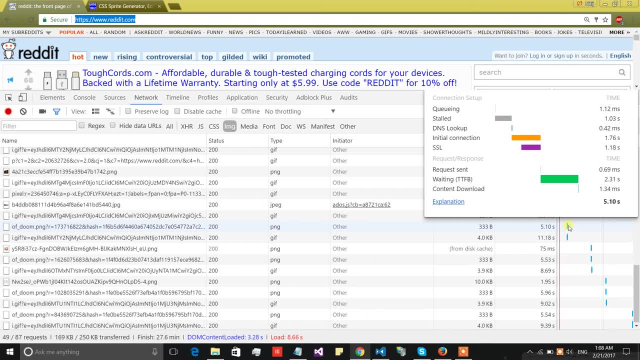 connection is secured or not. so this is a very simple way to download any resource or any component, and then the dtfb, or the time taken to time taken for first byte to arrive is much bigger than the actual download time. so, as you can see, it doesn't matter if the size of the resource is very small. 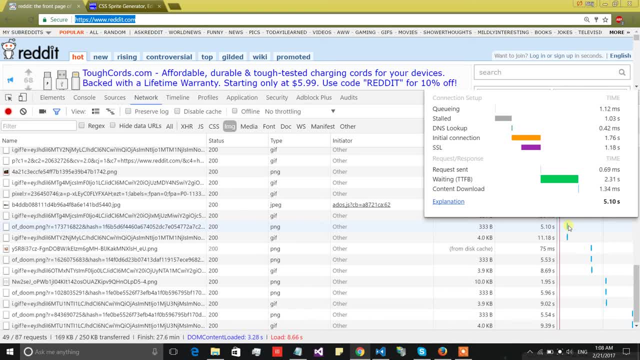 the actual download time is still going to be 5.10 seconds as compared to the 1.34 millisecond which is there, which is the actual time taken to download. so the total time is much bigger than the actual download time because there are so many different steps involved and you can see that the 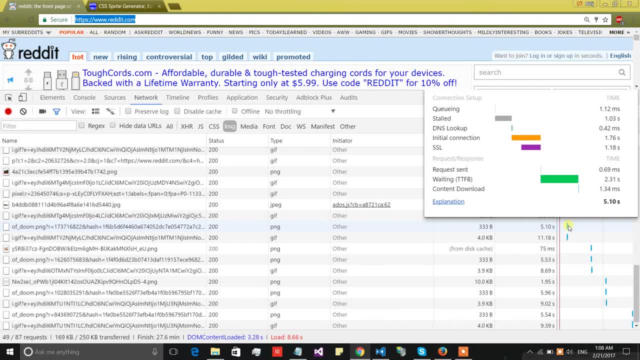 total time is much bigger than the actual download time because there are so many different steps involved. so as the number of smaller resources increase on a web page, the total time also becomes bigger, and this is the exact reason why large files take less time to download. so you can. 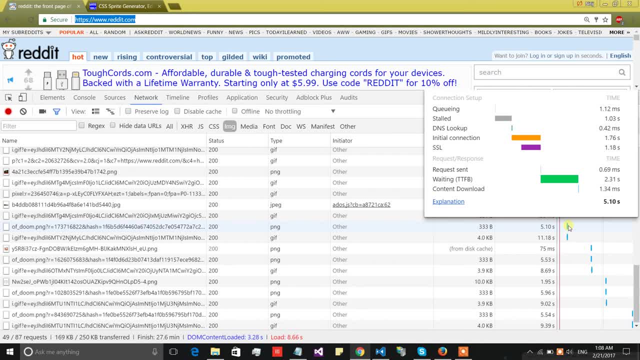 clearly see that the actual download time of the resource is not very much when compared to most of the item downloads. this clearly means that we should fix the problem which is bigger first, so as to get the maximum performance gains. improving the performance of the resource is very important. 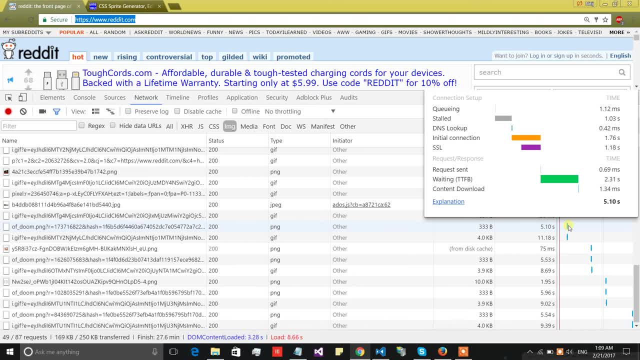 as to get the maximum performance gains. improving the performance of the resource is very important. download speeds will only take you so far, but improving time to first bite and dns lookup etc will be much more efficient. so now you know how little importance network speeds have when fetching a large number of small resources. all right, so now let's talk about the http request. 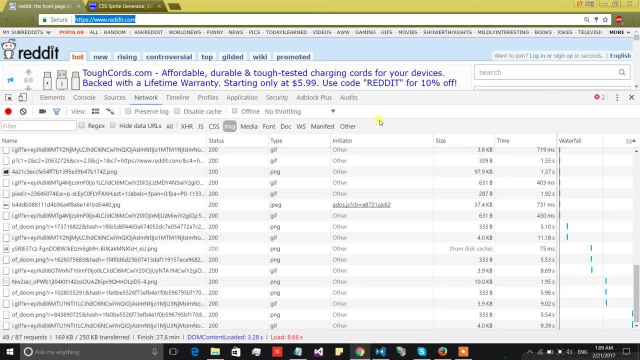 and network connections. the http request is composed of several different parts. first, the browser performs a dns lookup. after this, the connection is established. the actual downloading of the resource starts in the end. many times for smaller resources, the downloading time is much less as compared to other steps, as i discussed previously. so before the connection is established, 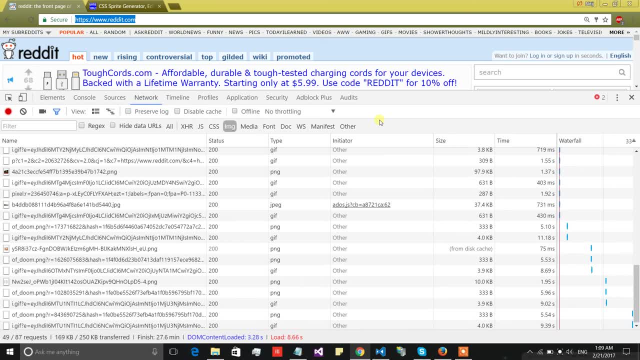 a three-way handshaking is done between the browser and the server. they basically agree upon how they are going to send and receive the data. when the first packet comes, then the browser may realize that it has the ability to accept more simultaneous packet and it tells the server that it. 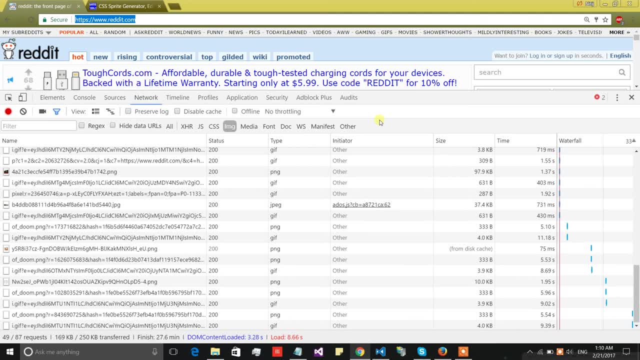 can do so, and this continues until a saturation point is reached. this is exactly why single large file will take less time to download than multiple files of a smaller size. then there are constraints on the total number of simultaneous downloads which are allowed by any browser. okay, now let's. 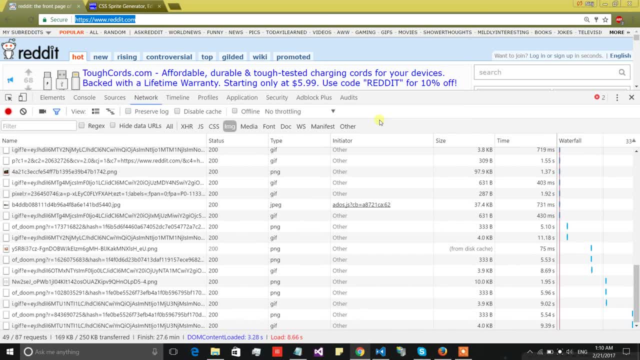 come to the script and style bundling, which is related to the number of resources on any web page. so if there are so many different scripts and styles being referenced or being included in the web page, then it is always a good idea to bundle them together, and we can do that for every kind of resource, but different kinds need different. 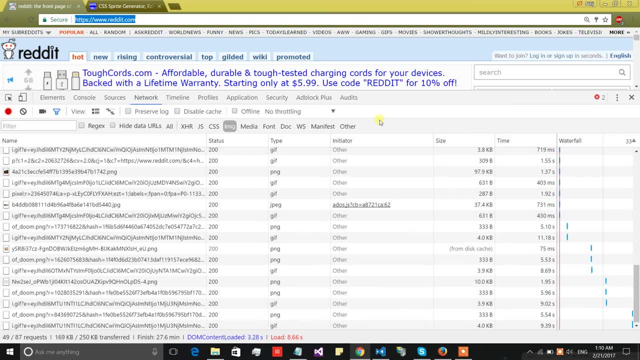 approaches to bundle. the script and css styles can be bundled by just concatenation in a single file. this leads to good performance gain. if there are numerous script and style files referenced in the web page for images, we need to follow a different approach which i will discuss in a 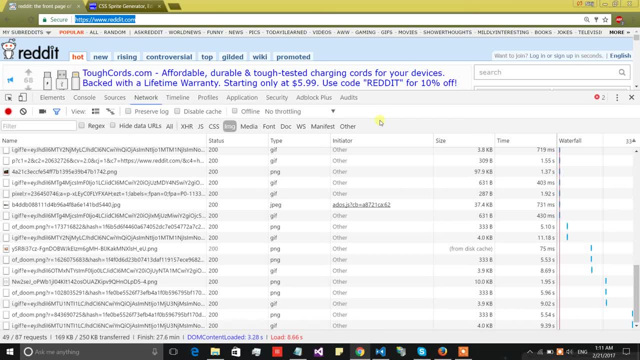 short while, okay. so oftentimes the browser caches the bundle file and it becomes difficult to make a script or a style changes and release new bundles, because the name of the bundle file is going to be the same. the solution to this, to this problem, is to attach a timestamp or version number with each. 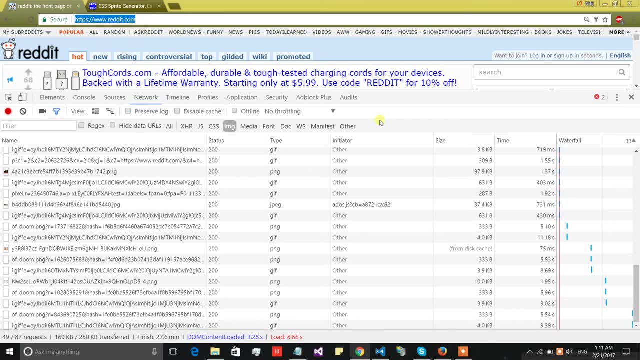 bundle file so that the browser will download the new content if there is any change in the name of the bundle file, instead of just fetching the old bundles from the cache. however, the thing to note over here is that then we would need to supply a new bundle for every little code change. a possible solution to 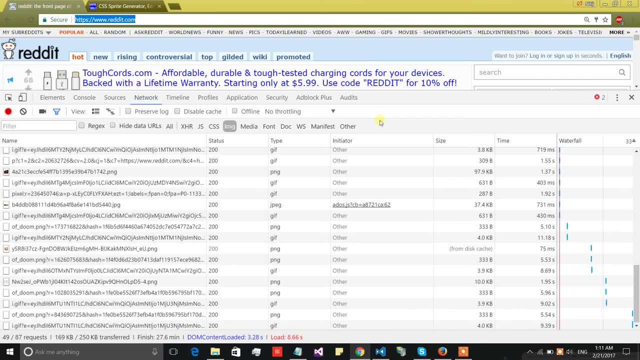 this problem is to create separate bundles for the library and the application code. so, for instance, if you are using jquery and angular, then bundle them together, because it is very unlikely that their code will change, but have a separate script bundle for the application code and also attach a 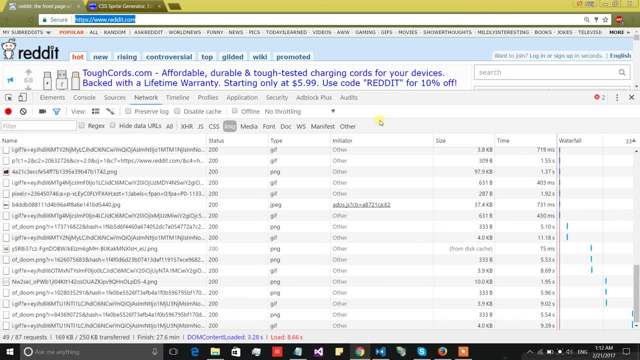 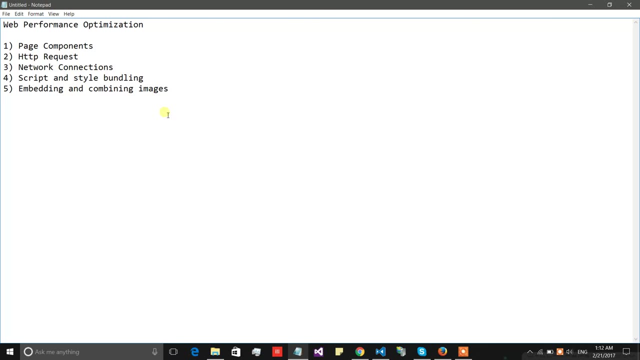 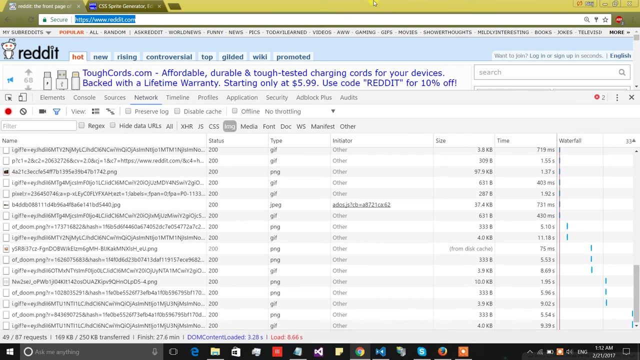 version number or a timestamp whenever you make a new build of your script code, and same could be done for the css styles too. so after this, let's come to the embedding and bundling of images, or combining of images so to concatenate images together. there are two popular ways in which. 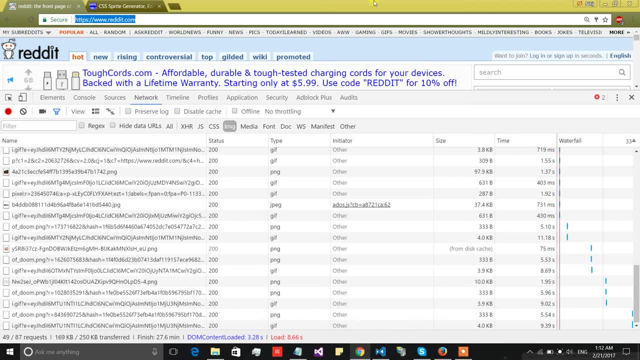 we can do that first. one is to embed them in the web page itself and then finally embed them in the existing page and then finally do the same with the other two images in place, so once we have all base 64 format. so base 64 format is basically used because we cannot use the binary characters. 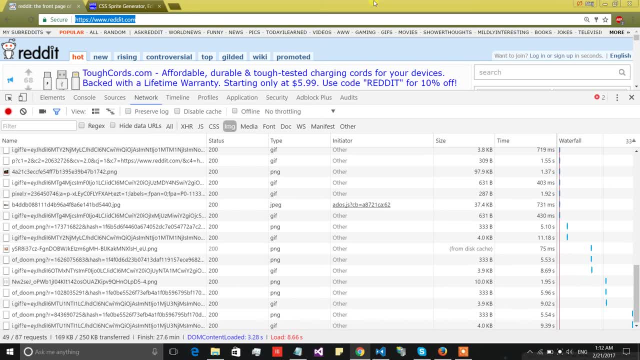 in the HTML page itself, and the other reason is that browsers are mostly all the browsers only supports the only support the base 64 format, so we don't have many options. the browser will download the images with the web pages as well, instead of opening separate connections to. 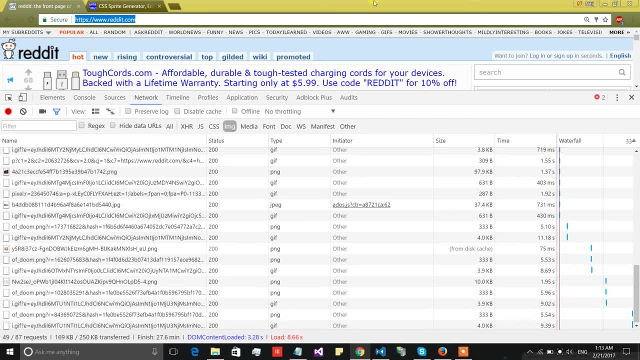 download them. this will result in good performance gains if there are numerous static images on the web page. if you want to load sets of images conditionally, depending on the user action and the currently opened view, then you can also use image sprites. so sprites are basically images. 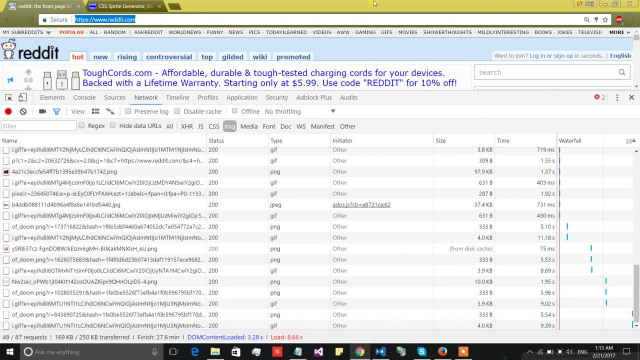 which are arranged in the form of a grid in a single image file. we can then use CSS to clip a specific part of that despite, based on the X and Y coordinates and the width and height of the image. so now I'm going to show you some code examples on how you can use the images sprites, as well as. 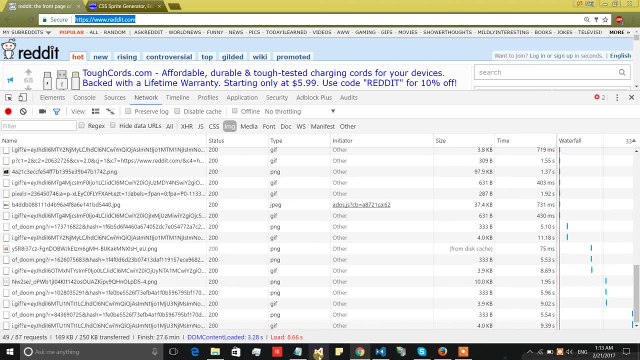 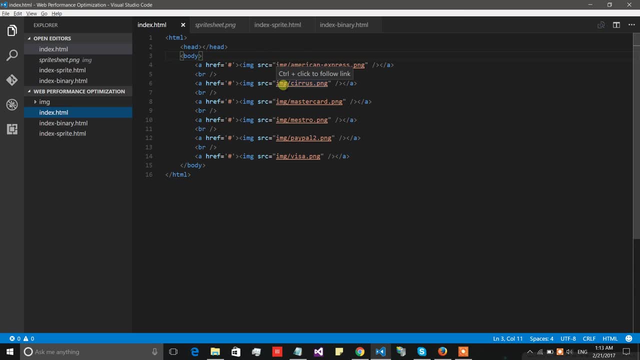 the binary image data inside an HTML page. so I have opened up the Visual Studio code and I have opened a folder as an application. so there is a indexhtml file and there is also a folder which is IMG, and inside the indexhtml file there is a folder called indexhtml file and inside the indexhtml 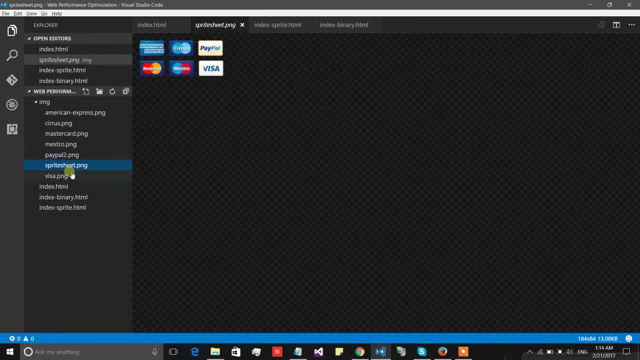 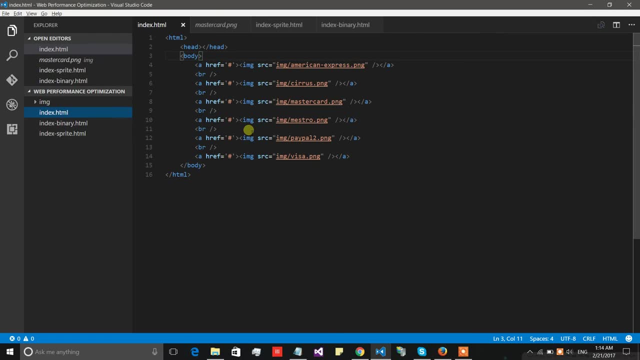 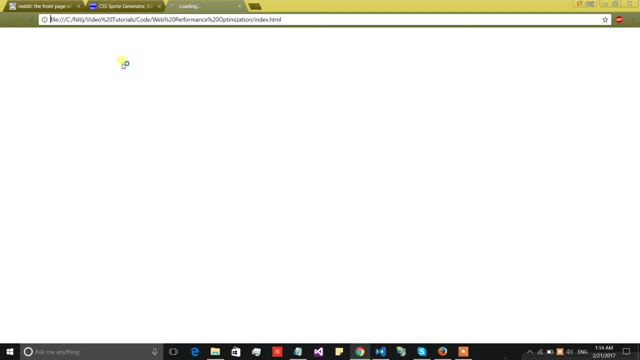 file it will be a wallet and inside this IMG folder there are several different icons for different kinds of payment systems, like there is the American Express and MasterCard etc. so in the first file, default indexhtml, I have added the anchors for all the different payment modes and if I run this indexhtml then we can see that they are all the anchors. 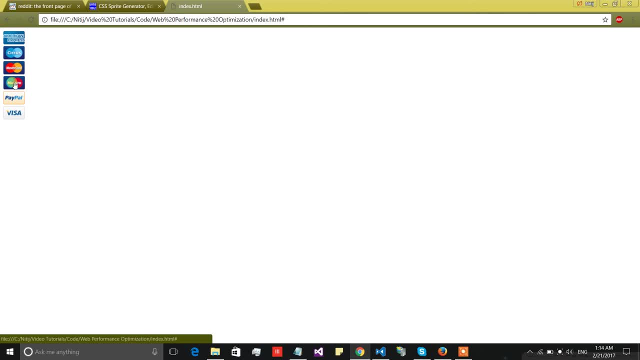 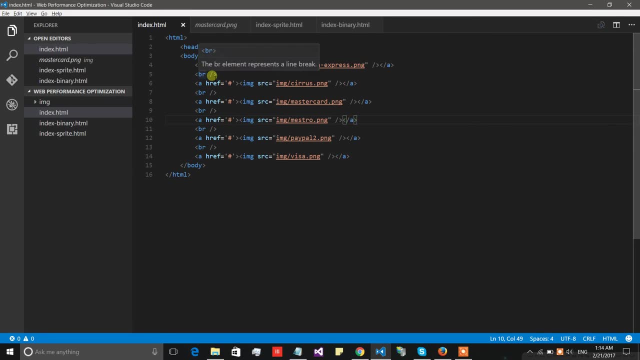 so these anchors are not actually pointing to anything, but still, you can see the images which we are getting from the img folder. all right, so if we have to convert or if we want to load all of these images in in in the, in the form of a single file, excuse me, in the form of a single. 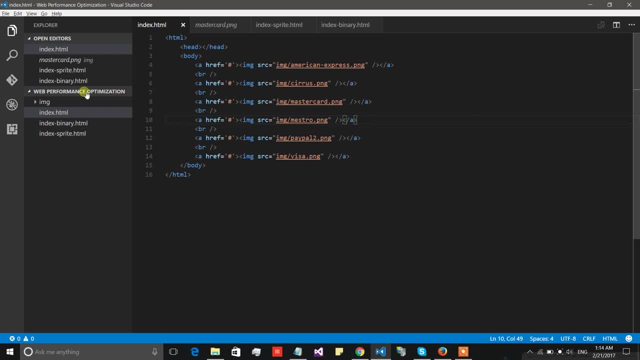 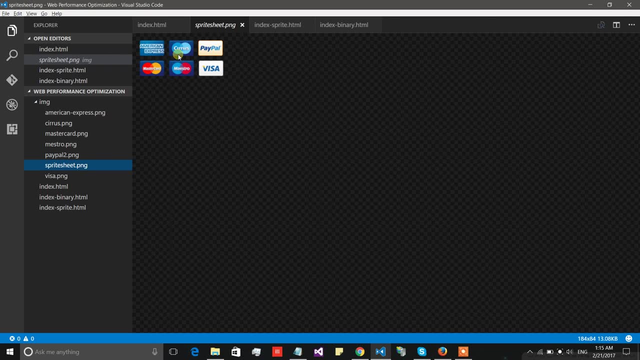 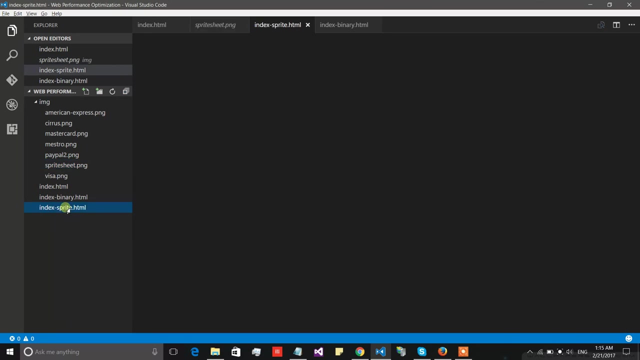 file. then we can do that using a image sprite, and i have already added a an image sprite and i will show you how you can create one yourself. and in this sprite there is a grid of all the different images. so in the web page, in this index spritehtml, there is a. there are basically classes. 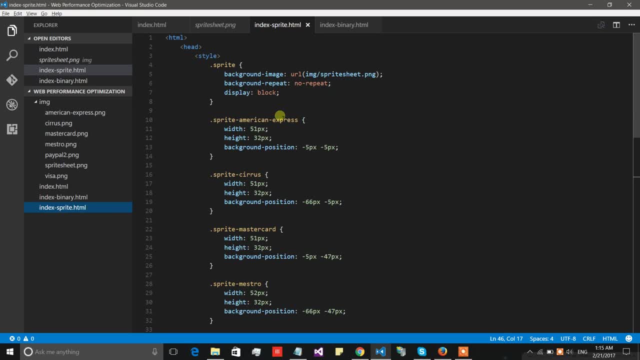 which are referencing this sprite image file. so, as you can see, this sprite class is is getting the the background image from from this path, and then there are individual classes for all the different payment methods, but inside them we have we have set the width, height and the background position for the x and y. 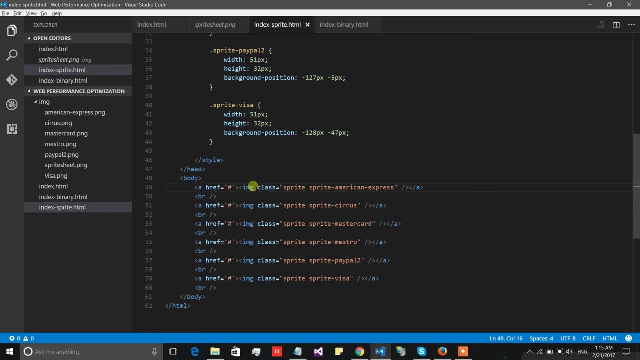 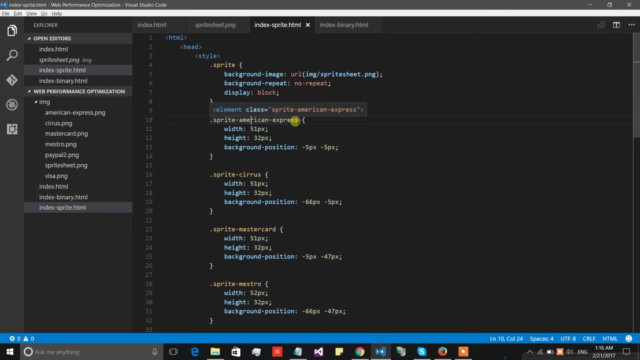 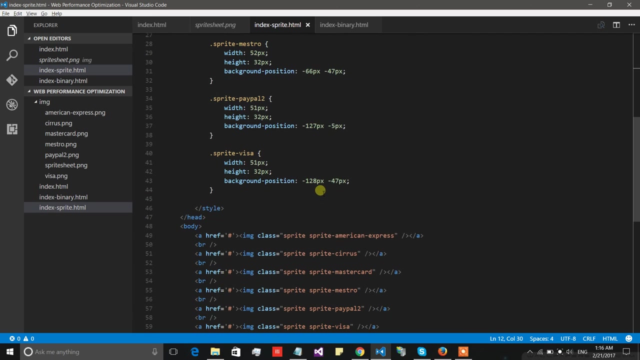 so now inside the inside the anchor links, instead of setting the source as a file name directly, i have set the class, so the class is now fetching the image and the individual classes are coming back, and so all the different payment methods are responsible for getting the exact image from the grid, depending on the width and height and the background position. 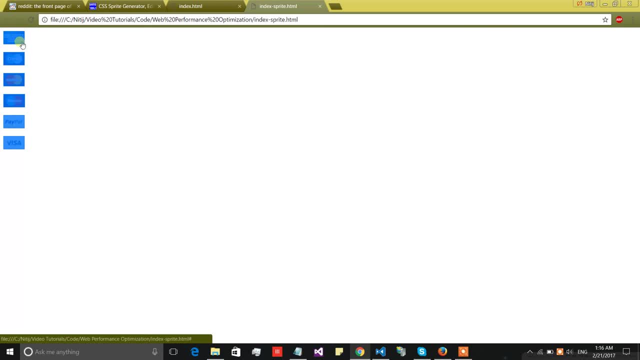 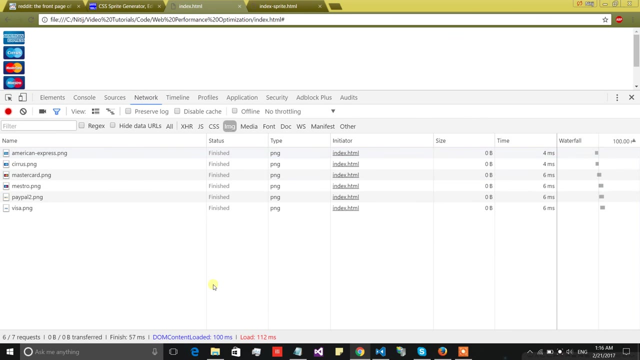 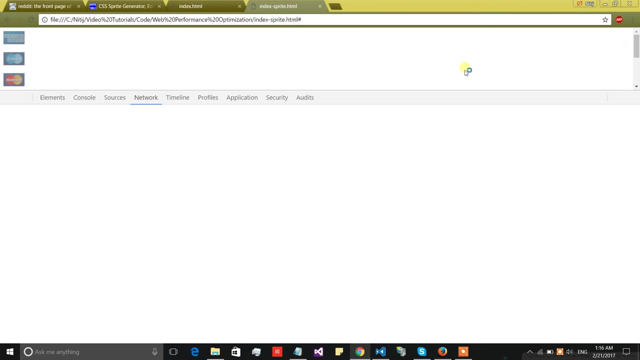 so if i run this index sprite then you can see. the result is also the same, but this time. and also let me show you how it is looking in the network profiler. so i have to refresh the page. so as you tab there are six requests. but over here in the profiler, if I am going to refresh the 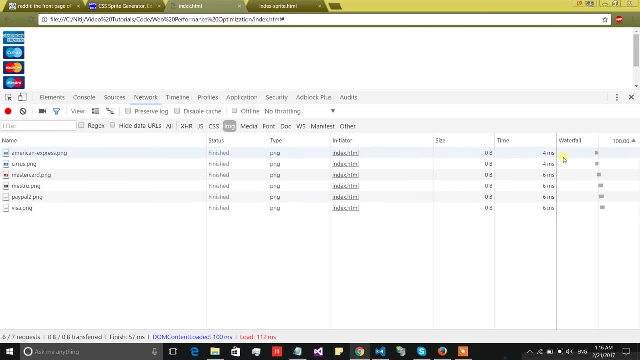 page. then you can see there is only a single request. so this entire, the all of the all of these requests are basically taking so much time, and over here only a single image is being loaded, which is very fast as compared to loading of six different images. okay, now let's. 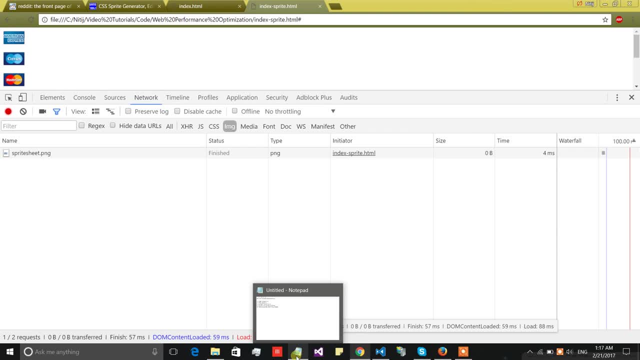 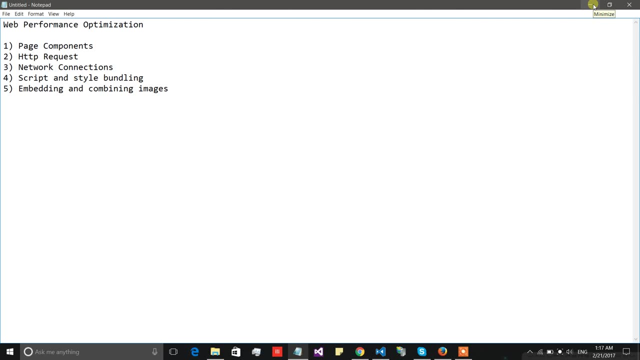 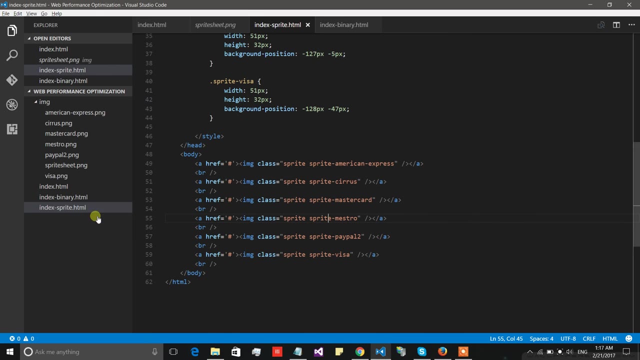 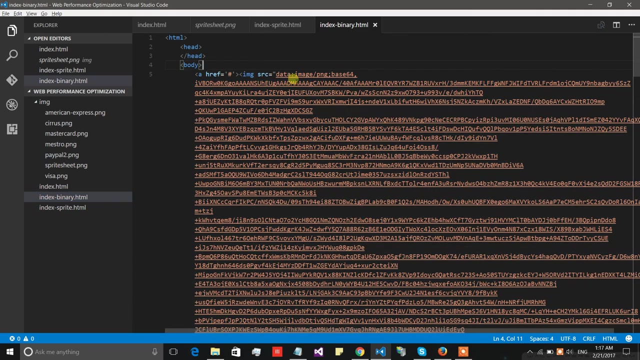 come to the way in which we can use the images as binary data and how we can embed them in the webpage itself. so for that we have to convert the images into the base64 format and then we can use the base64 value directly as the value for the src attribute for the image. so, as you can see, i have already. 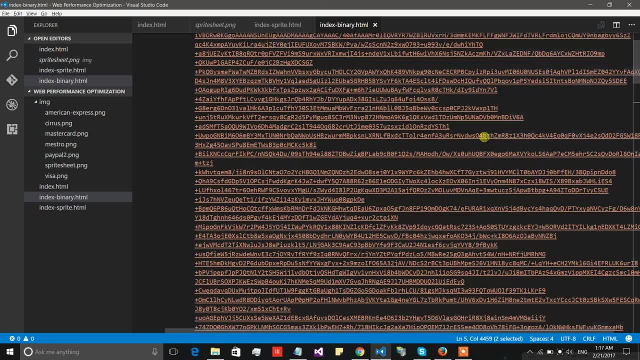 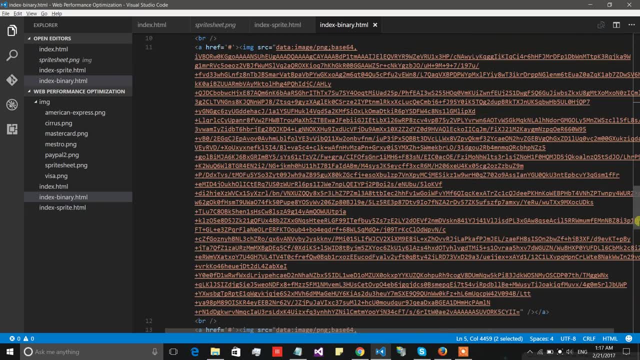 converted it. i will show you how you can do that yourself. basically, there are tools available online and you can select anyone which you think is suitable for you. so we cannot really make out which image is that. we can maybe put some kind of comments over here or some kind of.